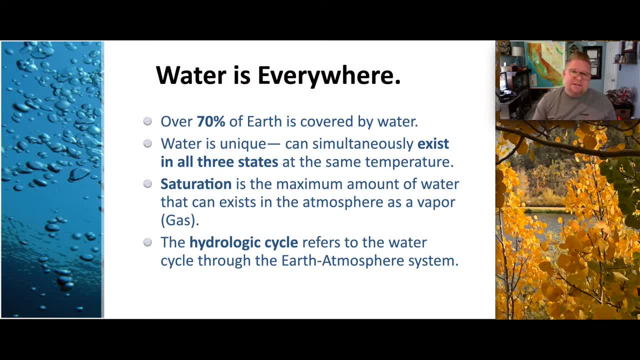 we'll use that word throughout this presentation. Saturation is the maximum amount of water that can exist in the atmosphere as a vapor. So when I think of the word saturation, I think of a washcloth, and a washcloth is 100% dry until you submerge it into water. 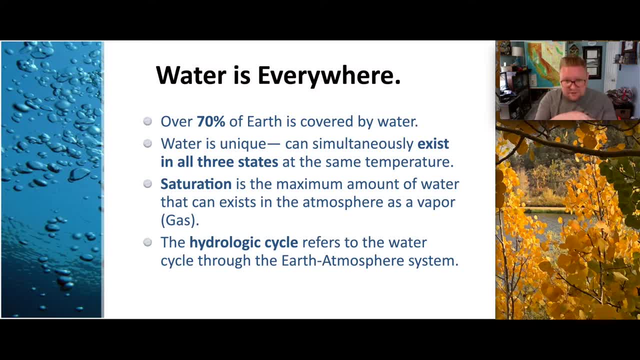 And there's, you know, different variables as to how much it can hold. but if you want to completely saturate, you can use a washcloth. So if you want to completely saturate, you can use a washcloth. So if you want to completely saturate, you can use a washcloth. So if you want, 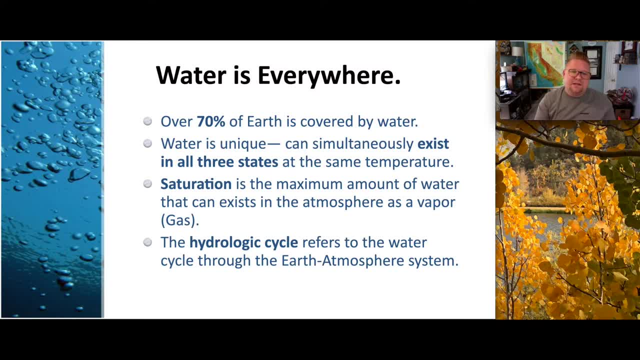 or make, you know, make that washcloth soaking wet. that means it cannot absorb any more water. It's at its maximum capacity and we'll call that saturation. So it's kind of that same idea. We'll also continue to use a lot of the terms from the hydrologic cycle, which 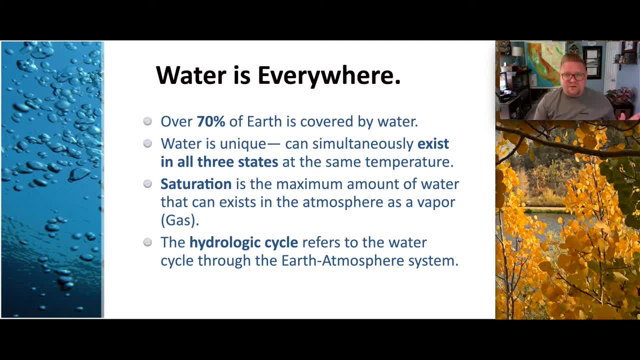 is something we've learned about at some point in, you know, elementary school and you maybe revisit it in high school, But we understand that there is a cycle in which the, you know, water will transfer through our Earth and atmosphere system, And we will make reference. 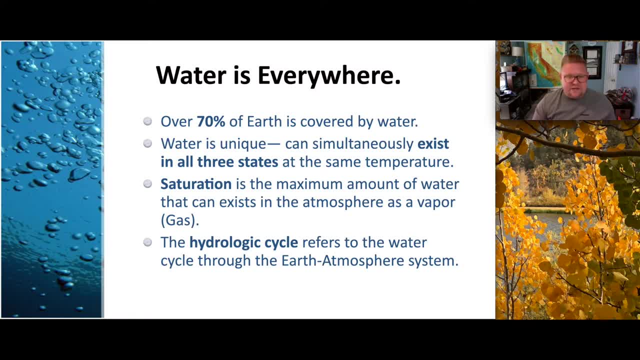 to some of that. You know, again, if you're going to do something like that, you're going- evaporation, condensation, precipitation- but there'll be others that we'll continue to mention throughout this and other presentations, such maybe as transpiration. You know, maybe you have. 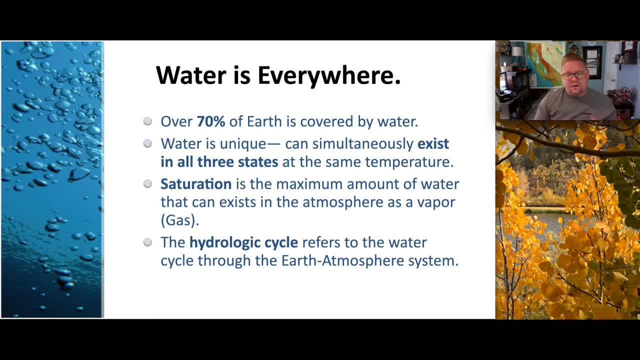 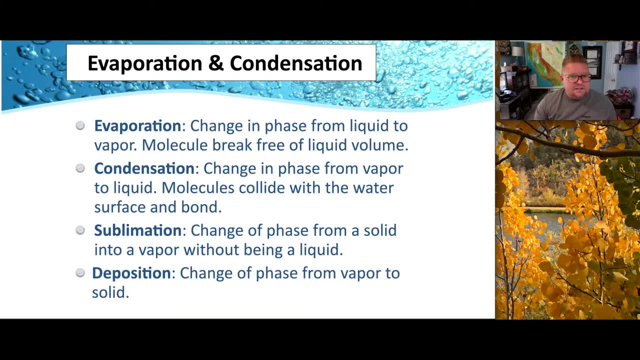 not heard of that term, and so we'll continue to expand on the complexities of the hydrologic cycle. Now, to move forward, let's mention a couple different. you know the elements, the ones that we are familiar with within the hydrologic cycle. We have evaporation, which is the change in phase. 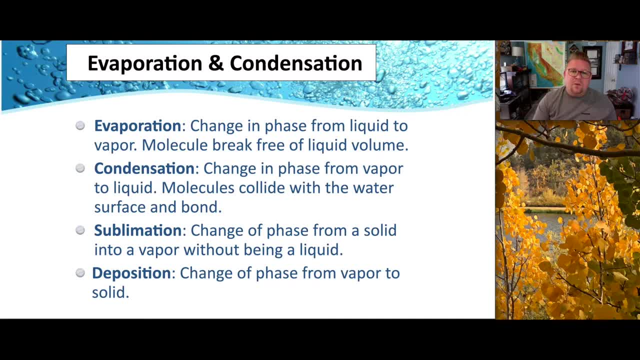 from a liquid to vapor, The molecules break free of liquid form. We also have condensation. You know, condensation is a great example of you know, if I have my iced tea here, if I had, if the contents in the glass were colder than the surrounding air, condensation would, you know, accumulate on the 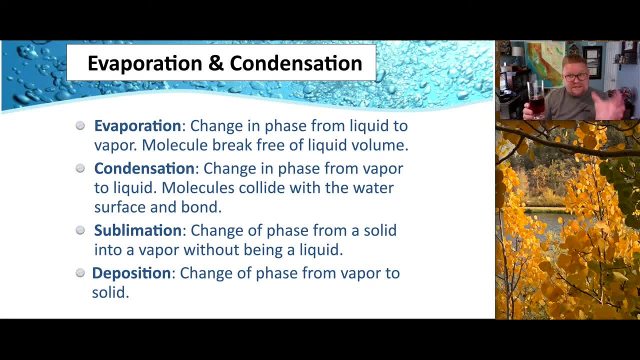 outside of the glass, because it would be pulling in the moisture that's in the air and adhering it to the glass and then it would then condense and turn into droplets, which is again a change in phase from vapor to liquid. Sublimation is probably something you 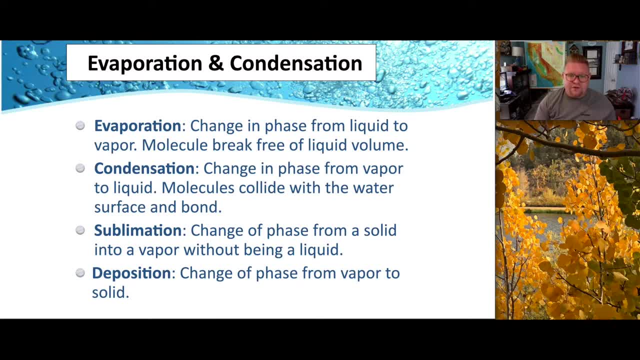 have to think about a lot of times, because it's a very, very important thing to think about. haven't heard of. and also deposition. So sublimation is the change of a phase from a solid directly into a vapor without becoming a liquid, and deposition is the opposite of where a vapor 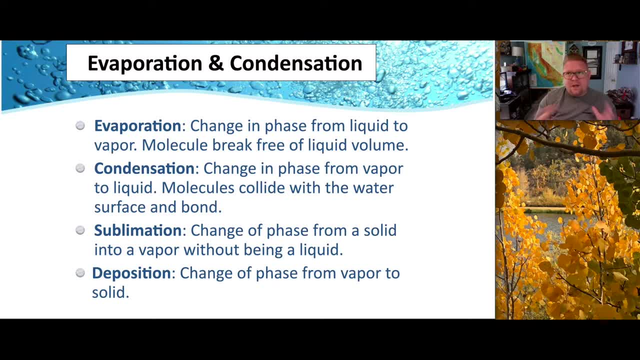 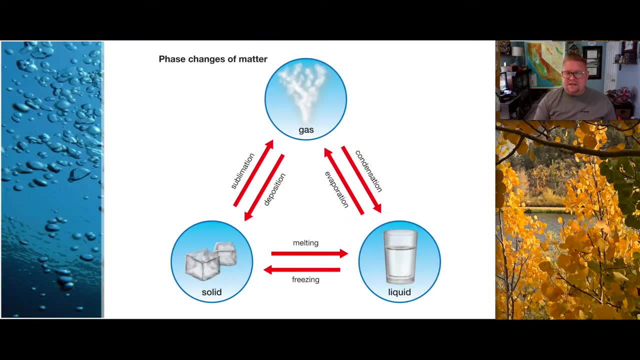 will immediately turn into a solid and, will you know, it kind of bypasses the middle person right, It bypasses the liquid state, and so those are extremes, but they do exist and we'll continue to talk more about that in this and other presentations. So let's look at the phase changes. 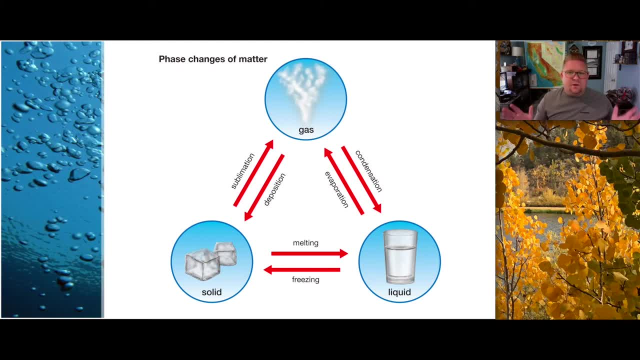 of matter. So, again, something that we've all seen before and that's awesome. you know, you've got solid liquid and you've got gas. We also then have the term that's mentioned from going from one to another. So, again, if we're going from perhaps a gas to a liquid, a condensation, 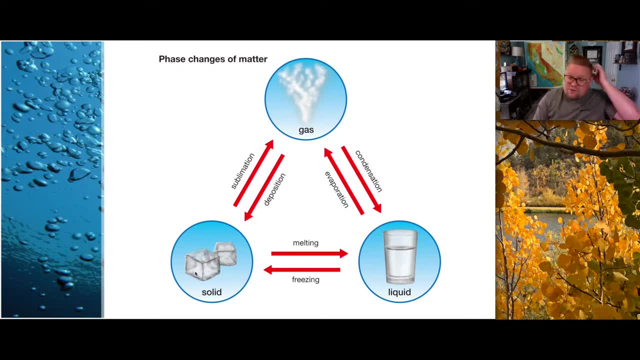 will occur. If we're going to go from a liquid to perhaps a solid, we'll see that freezing is going to occur. But something that we need to take into consideration when looking at this is not just the phase change, which is identified within these terms, but to think about the energy or the heat that needs to be either 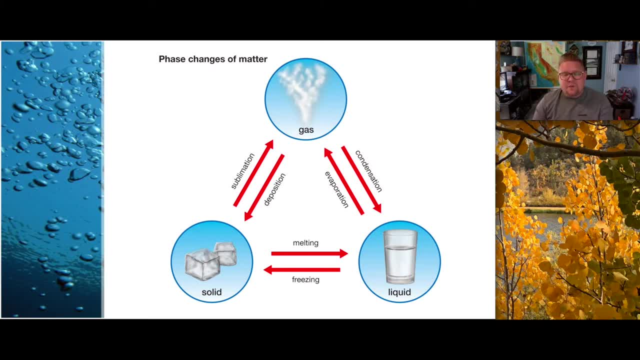 absorbed or released in this process. So, as an example, you know, it's a hot summer day, we're outside and we begin to perspire or we begin to sweat, So we have produced a liquid on the outside of our skin. Well, that liquid evaporates, It goes into a water vapor and goes away. Well, 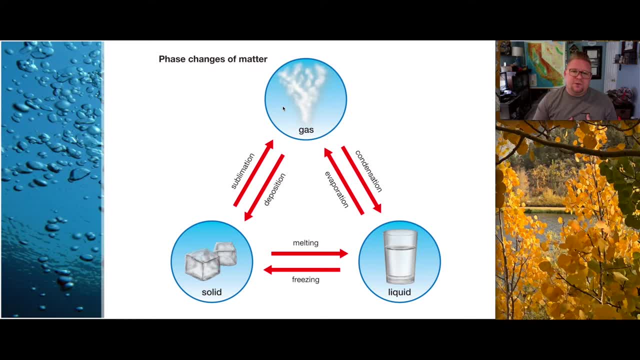 why do we do that? Why does our bodies, you know, go through that process? Well, when the liquid is present, the energy, you know, within our atmosphere, the temperatures from your body and the heat around will cause that water droplet to evaporate, turns into a gas and it goes away. But in 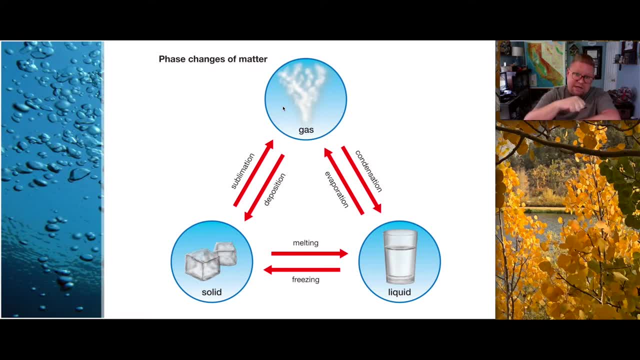 that process, heat is going to be absorbed within that water molecule, which will turn it into a vapor. So heat is being absorbed and then, in that, you know, as it absorbs, it takes it away as a vapor. Well, if you take the heat away, what happens to the surface? 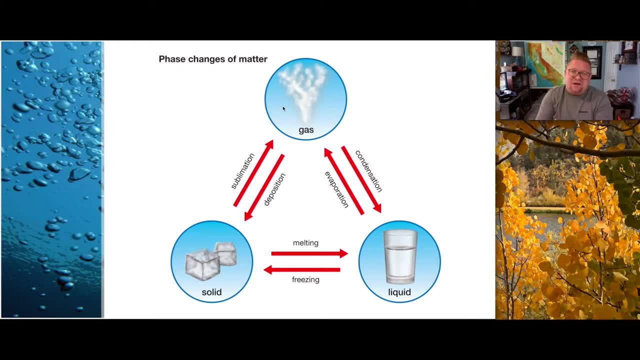 of your body. Well, you begin to cool down because you're left behind, you know, with a cooling effect Because the heat is being absorbed and taken away. So that's an example of that. But what if we wanted to go from, say, a liquid into a solid, Like you know, from a glass of water? 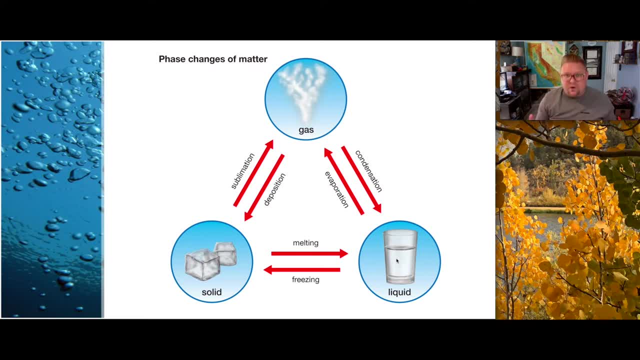 into an ice cube. Well, you're going to need to remove all of the heat, So you're not going to be absorbing heat. The liquid will not be absorbing it. It has to release it. It has to let so much go that it's going to be able to freeze. So that's something to 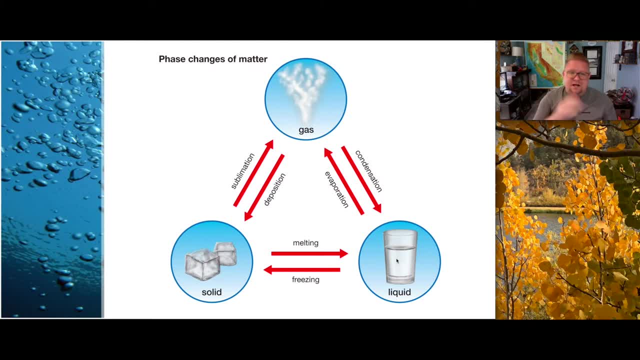 take into consideration when looking at this diagram as we continue to work through the process. So that's something to take into consideration when looking at this diagram as we continue to work through the process. So that's something to take into consideration when looking at this diagram as we continue. 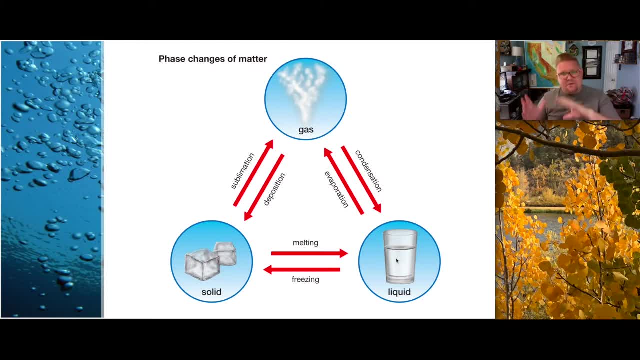 to work through the process. So that's something to take into consideration when looking at this diagram, as we continue to talk about the phase changes of matter, Is that sure? what is the name of the process? Is there melting, freezing, condensation, evaporation? That's. 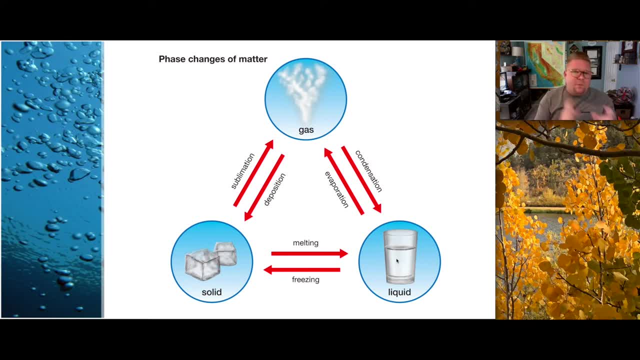 great. But also, in the back of your mind, think about, well, what's happening with the energy that you know. again, we may not be able to see it, but we know it exists. Is this going to be an absorbing or a releasing factor? And that really helps paint the picture. 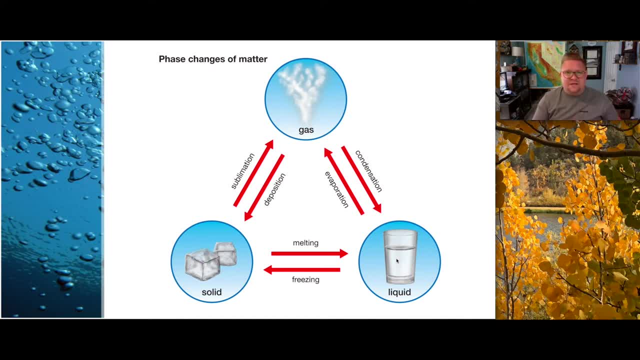 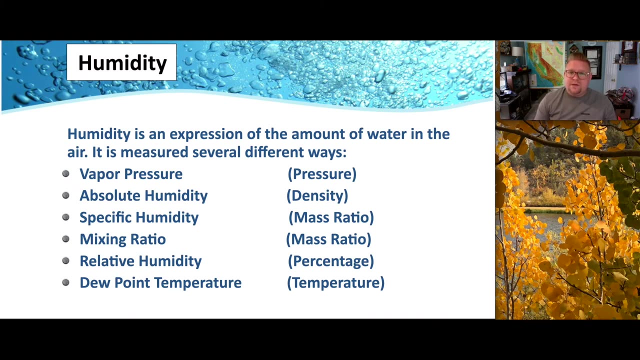 later on when we talk about different you know things- thunderstorms and lightning and stuff like that, talking about this latent energy that could be stored through these processes. so then let's move on into the term humidity. so humidity is an expression of the amount of water in an air. 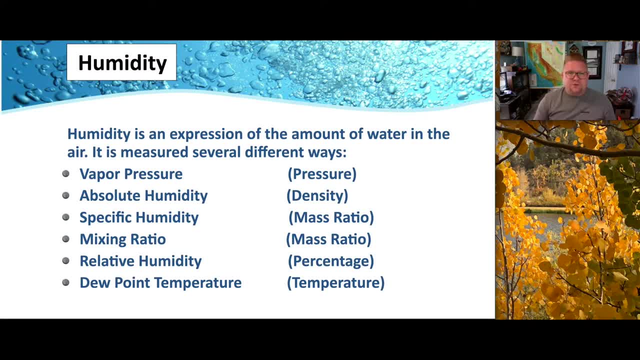 parcel or the air. so you know an air parcel just means a measurement of air. so, like my office that i'm in, i could identify as being a parcel of air. obviously, in you know the atmospheric world we talk about much larger parcels, but that's just an example. it is measured many different ways: the 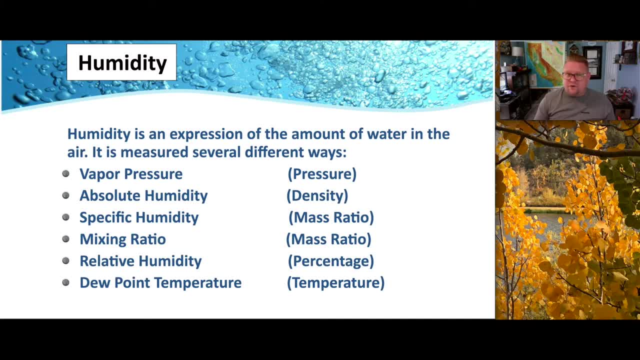 humidity. we can look at it, you know. we can measure the vapor pressure, the absolute humidity, the specific humidity. we can identify a mixing ratio, we can talk about relative humidity and dew point temperature. so these are all terms that we can look at when measuring humidity. so you know it's. 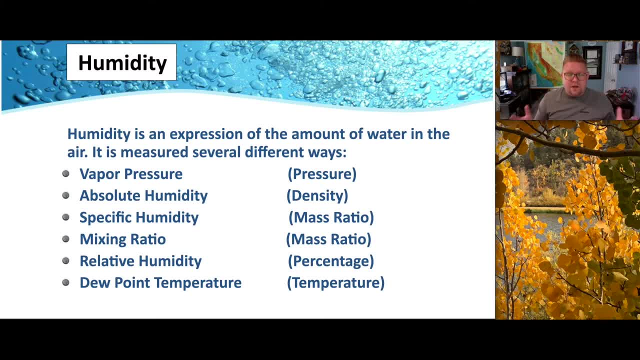 very broad, you know, or an umbrella term with a lot of different elements that kind of go into it. it. so what i've done here first is i provided the term, you know, vapor pressure, which is we're going to identify the pressure in that parcel of air, which helps us understand more about the humidity. 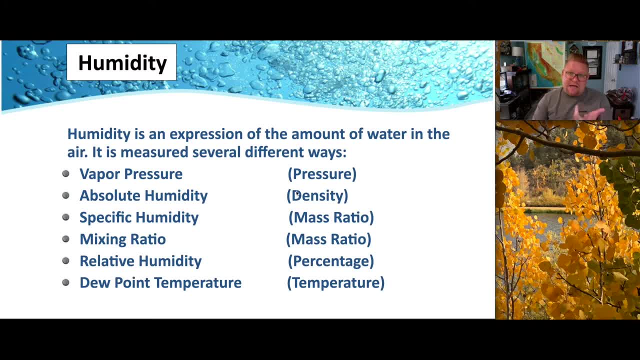 we want to look at the absolute, or the density of the actual water in the air, the mixing ratio, which is the mass ratio. within this, both specific humidity and the mixing ratio, we'll also look at the relative humidity as a percentage and dew point temperature, which is essentially the 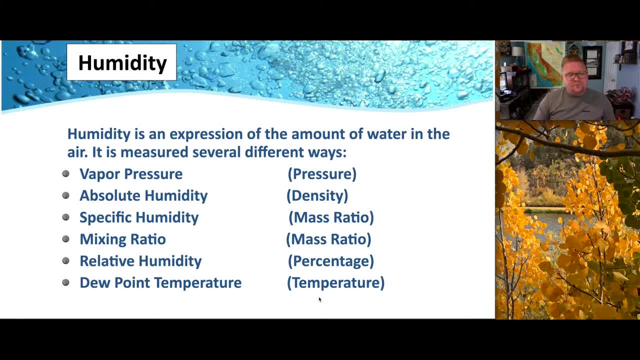 temperatures that are involved in order for condensation to occur. so what i want to do before i mean i know this is a lot right here. i actually broke this down a little bit further into groupings, so let's talk a little bit more about humidity and these- i you know these very specific six terms. 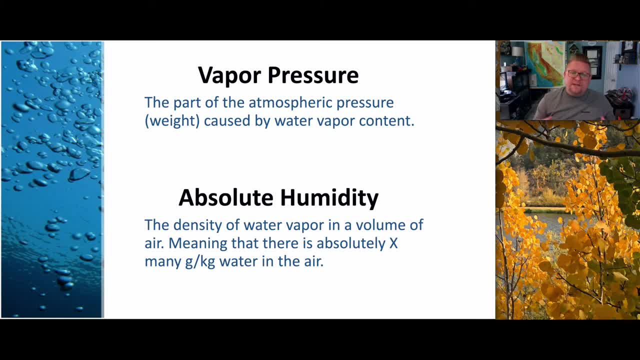 that i've identified here. okay, so what is vapor pressure? well, it's the part of the atmospheric pressure or the weight caused by the water vapor content itself. so we know that moisture water itself has density, it has weight, and we know that. you know what is almost. 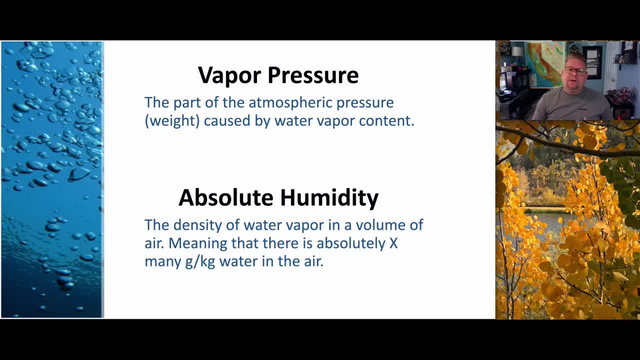 a gallon of water weighs a little over eight pounds. so when we can look at the vapor pressure, you know, based on how much water, vapor is in that parcel, will add additional weight which will then push down onto the surface, which is measurable. another term we have here is absolute humidity. 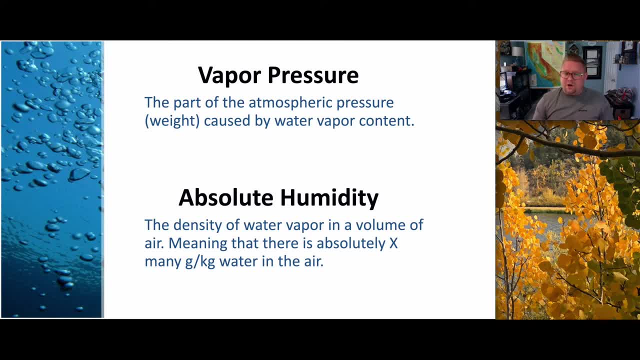 so the density of the water vapor in a volume of air, meaning that there is absolutely x grams per kilogram of water in the air. so what does that mean? so if we were to measure the weight of the air parcel, how you know, in kilograms how many grams are of the water? so as an example, i 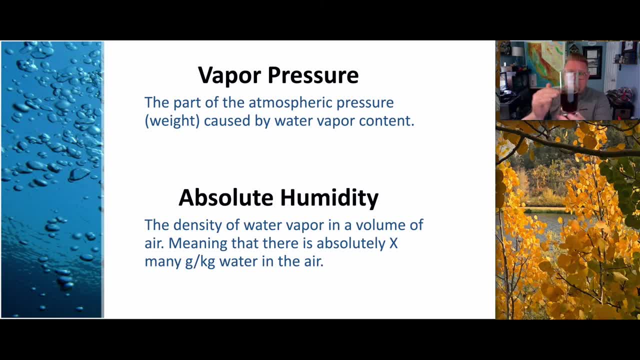 go back to my glass of iced tea. i can measure. there's absolutely- you know this- many grams per kilogram of moisture or tea in my glass. you know, i can give it a measurement. so in this case it's a 16 ounce glass. there's exactly eight ounces, so i know that it's absolutely 36. 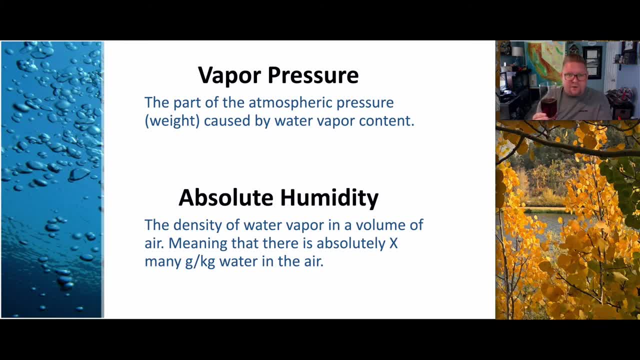 an absolute number of moisture, of measurable moisture. that's in there and that's really important for us to know, because I guess I'll kind of don't break into it, we'll talk about in a moment. then, when we get to the word relative humidity, that's a relative, relative means ratio or percentage. so I could say: 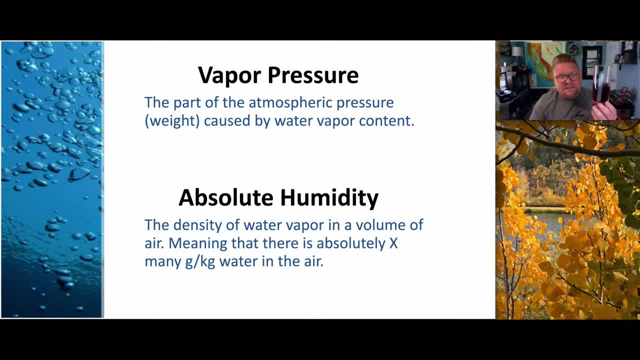 that, yes, there's exactly eight ounces of iced tea in this class, but I could also say that it's 50% full. so I can look at two different ways of two different sets of numbers, but still essentially mean the same thing. so we also have a term. 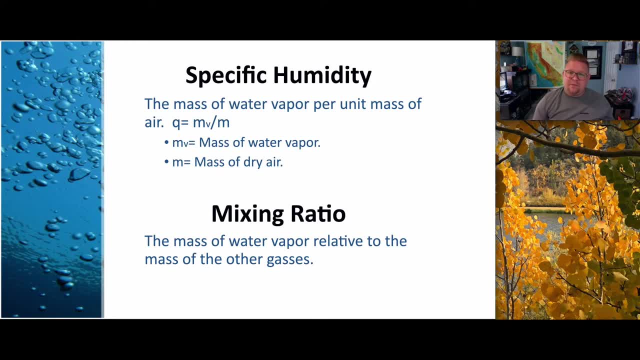 called specific humidity, which is the mass of water vapor per unit mass of air. so it's measured. you know specific humidity is going to be Q. Q is equal to the mass of the water vapor divided by the mass of the dry air. so you're comparing the mass of the water vapor versus the mass of the dry air. it's very. 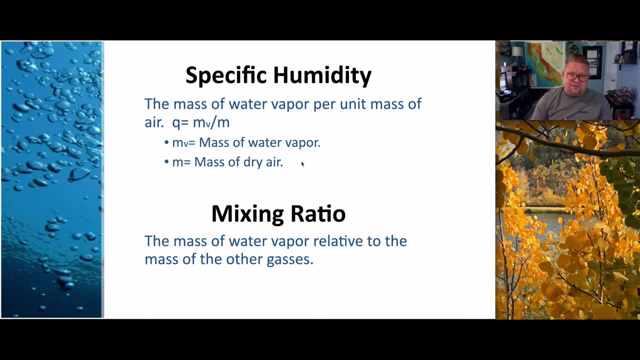 similar to absolute humidity, but this gives us an absolute humidity actual percentage. The mixing ratio is the mass of water vapor relative to the mass of the other gases. We'll also begin to look at the mixing ratios a little bit differently as to how much. 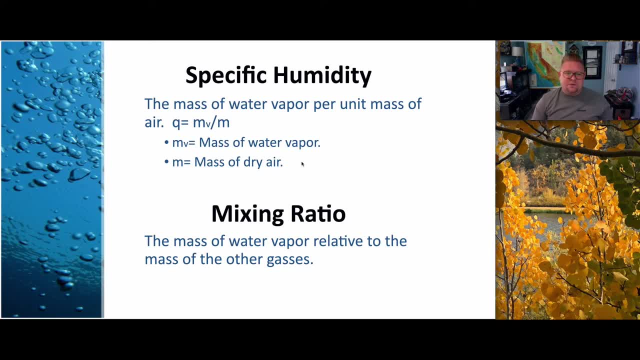 is the maximum amount of water that can be held. but in this case what we're trying to identify within the mixing ratio is: you know the mass of water vapor compared to what other gases are available in that parcel, or you know measurement of air? Then we can move on into relative humidity. 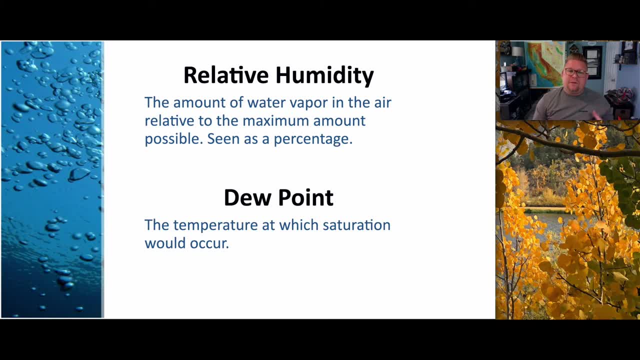 which I mentioned, which is the percentage. It's the amount of water vapor in the air relative to the maximum amount possible, seen as percentage. So you know, if this glass is a maximum of 16 ounces and it has eight, so it's therefore 50 percent full and that would be your relative humidity. 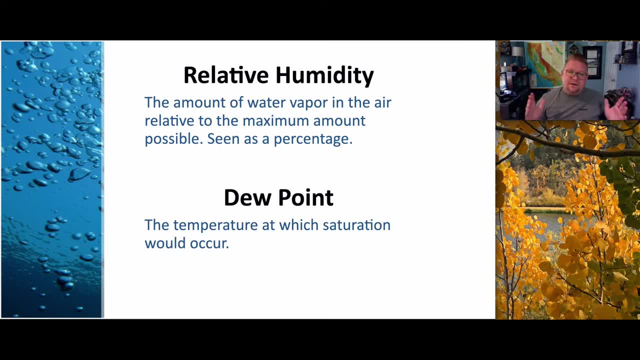 And as we'll learn- and we have learned that you know, the temperature of the air will regulate how much moisture will be able to be within it. We find that warmer air has the capacity to hold more water vapor or water content. Technically, the air isn't holding it, but as the air molecules, 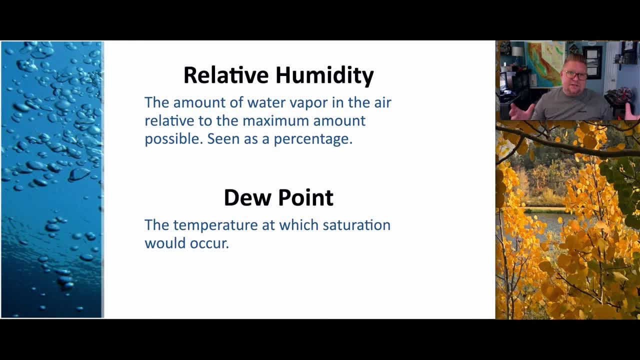 get you know, spread out because it's warmer air, it has the capacity to allow more vapor to be present. And then the last term is going to be our dew point, the temperature at which saturation would occur. So, essentially, when we think of dew point, is it what temperature is needed for? 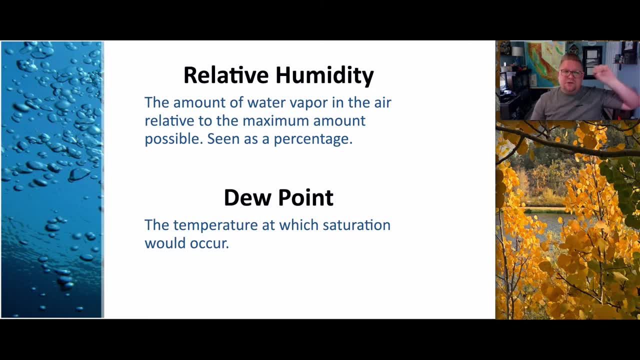 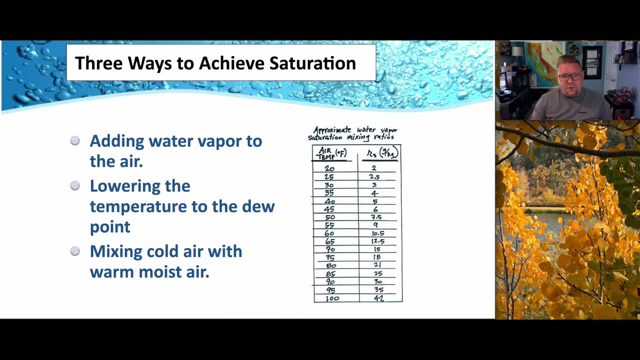 you know, the invisible gas that is there to become visible. you know, as you know, perhaps as precipitation. So what temperature is needed for that to occur, And that is a measurable element, as we'll talk about at some point later. So, moving forward, we can look at: well, how do we? 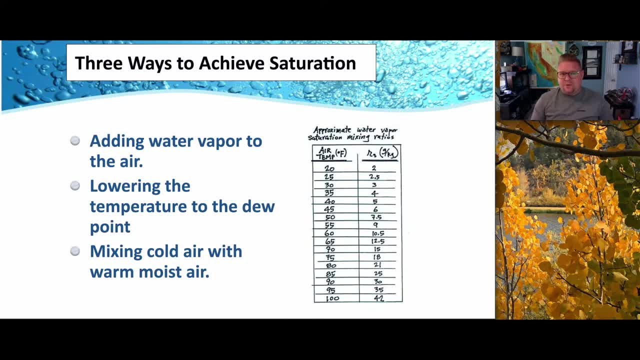 achieve saturation. Well, there's three primary ways in which we can achieve saturation, or how the atmosphere around you can be at 100 percent. You can either add water vapor to the air, you can actually lower the temperature to cause greater humidity and then to reach dew point And we 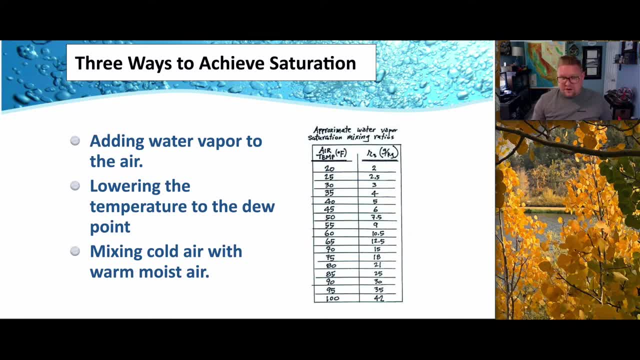 can also mix cold air with warm, moist air in much ways that a lot of our storms and extreme weather will do. So there's three ways to achieve saturation. I've also included this little chart on the right to just kind of- I mentioned it already, but to kind of bring it more into fruition is that 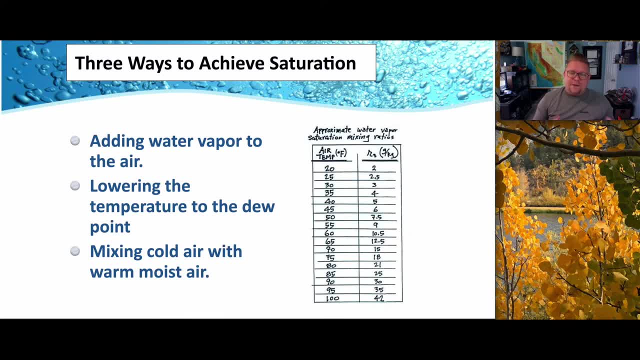 the warmer the air, the greater the grams per kilogram of water can be held. So, as an example, if we look at this table here, you know, at 25 degrees Fahrenheit it has a maximum of 25 grams per kilogram of air. That's the maximum that can be held. 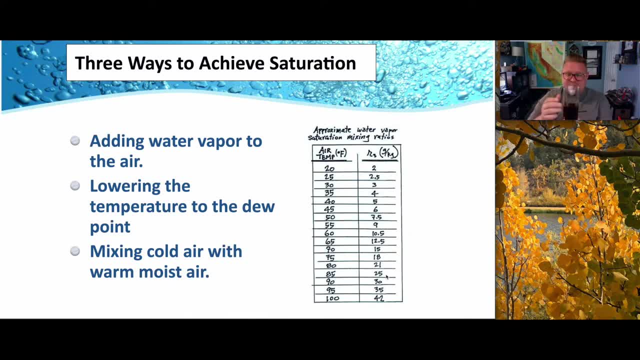 So again, you know, looking at this glass, the maximum that can be held would be, say, 16 ounces. So that's the maximum. So anything less than that is less than, and we can divide those two to get a percentage. So this is a. 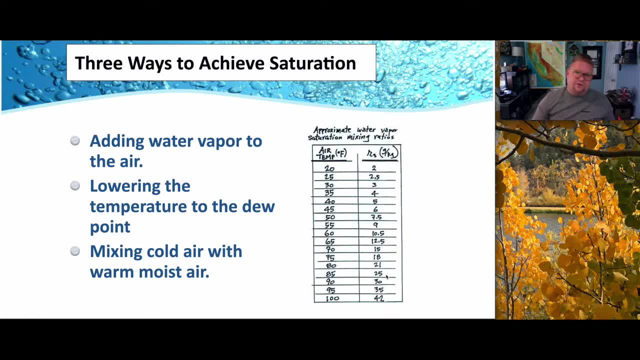 different way to evaluate, you know, humidity, moisture and our atmosphere. Now I've we've been dancing around it, So let's see what that looks like. So let's see this in action. So what would that look like? So I use this example because I think it's probably the 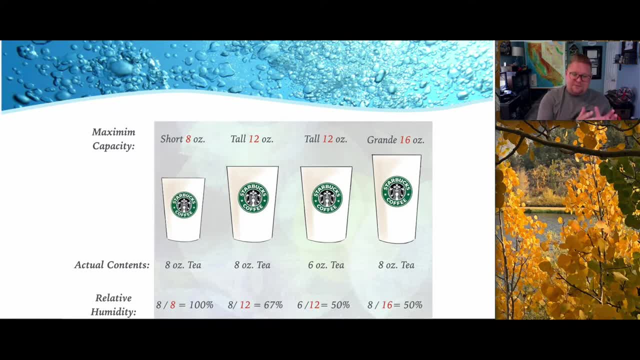 easiest is that we have, you know, this idea of maximum capacity. We'll also have this idea of absolute or actual content, and between those we use the relative humidity. Now, I'm sharing this because we'll continue to work through this. 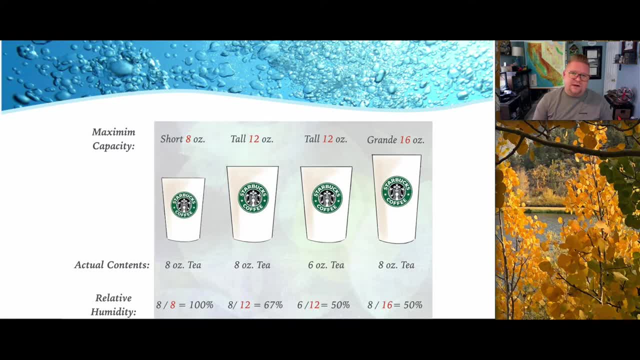 throughout these videos. but relative humidity is the phrase that you hear the most When you check your phone in the morning and it's like what's the weather going to be like? and it gives you a percentage: Oh, it's going to be. 85 degrees and humidity is going to be around 55 degrees if you do a percent rather. So what does that mean? Because you know a 50% humidity in California can be felt very differently than a 50% humidity, say, in Florida. And why? 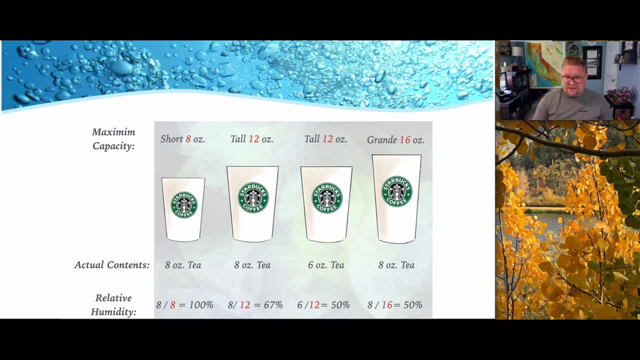 Why does it feel different if it's the same number, And I'll be able to explain that here. So we all know of Starbucks, right, And they have three cups. They've got the short, a tall and a grande. 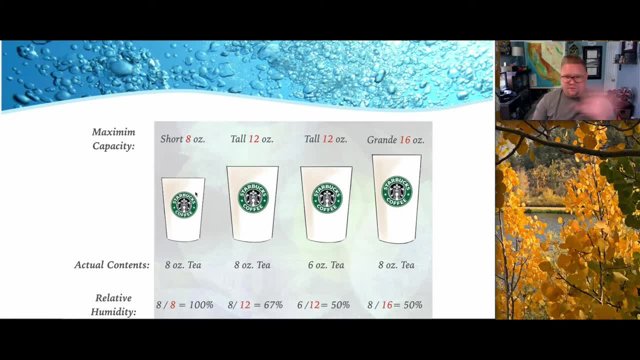 So a short, you know, and I don't know if these numbers are actually accurate, I'm just using it as an example. We'll say that the short holds 8 ounces, a tall holds 12, and a grande holds 16 ounces. That is the maximum capacity. 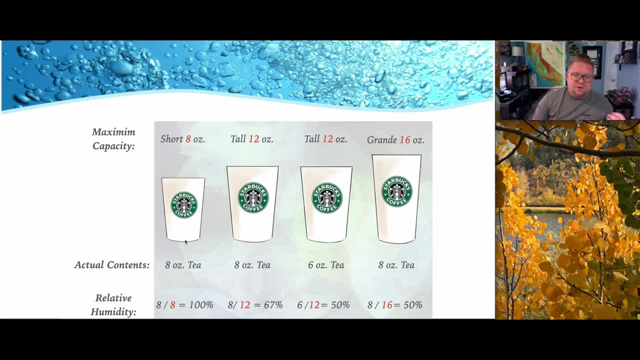 of between these three types of cups. So that's the maximum. Well, what is actually in it? Well, let's say that I have a short which has a maximum capacity of 8 ounces, and it has 8 ounces. 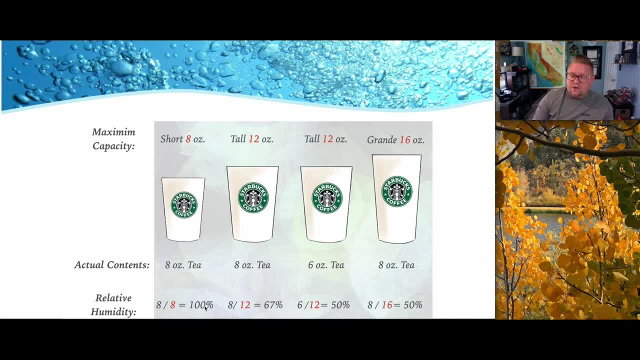 8 divided by 8 equals 100%. It's full. But what if I take my 8 ounces and I just pour it into a tall cup? Well, now it has 8, but it could hold 12, so it's only 67% full. Well, you know again what if I take a tall that could hold 12,. 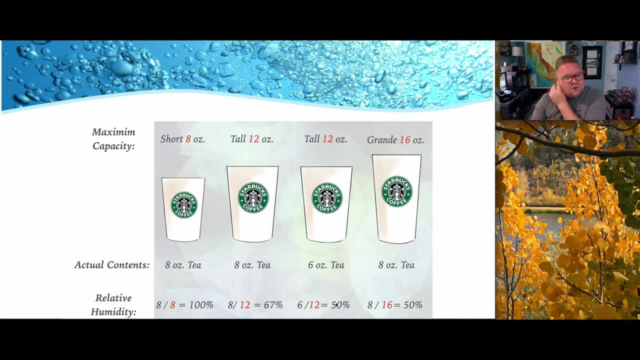 but I put 6 in it. Well, now it's only 50% full. So the reason I'm showing you this is because, look at these last two, You have a tall which is 12, and a grande that is 16 ounces. okay, Two different size cups. 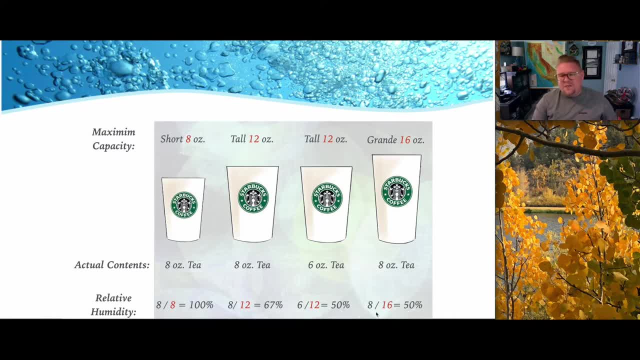 But notice down in here that as a relative humidity they're both at 50%, But this one only has 6 and this one only has 8 ounces. This one has way more. This 50% full cup has more than this 50% full cup, doesn't it? And that's because the cup on the right 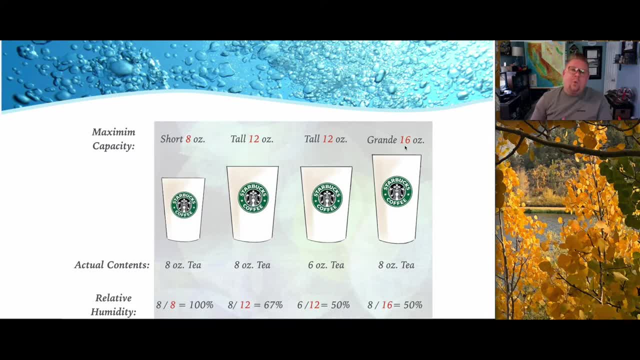 the grande is larger. So what we find in this instance? let's compare California to Florida. This would be California. This would be California be Florida. Florida can be significantly warmer, which means it could hold more water, which means 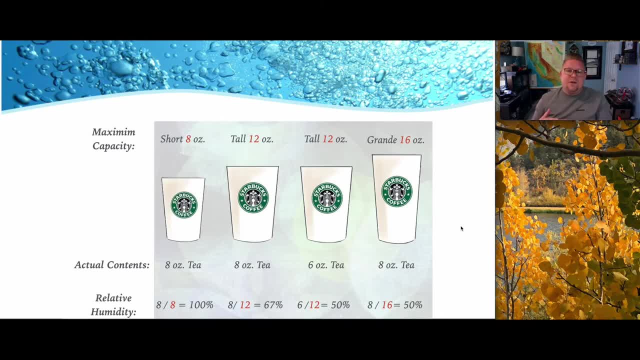 it could have a higher humidity, which means that you know if it's- you know- 80 degrees and 50% humidity in Florida, that is going to have more moisture in the air than California. that maybe is 60 degrees and you know, with 50% humidity It's a smaller cup, it's cooler air so it holds less. 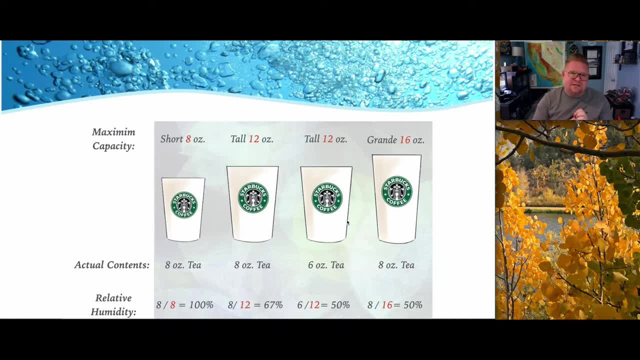 So I hope that kind of helps distinguish the differences there, because people are like, oh my gosh, like why, you know why is Florida? it was almost the same temperature but it's way more humid and it's well. it's because it is essentially it can be similar, but they have a 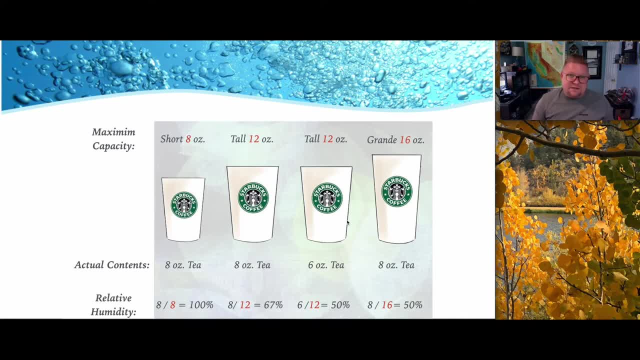 lot of different elements that we'll talk about later, But I mean the fact that it's a peninsula, it's a massive peninsula and it has water. it's a lot of different elements, it's a lot of different water almost all the way around it, So it's going to have, you know, generally more evaporation. 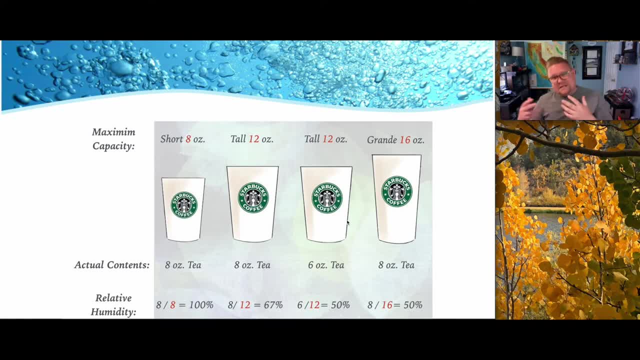 available, which means you're going to add more water content to the atmosphere anyway, So you're going to have higher humidity anyway. but then it gets really warm out there as well, because it's closer towards the tropics, And so it continues to get warmer, warmer, warmer, and it 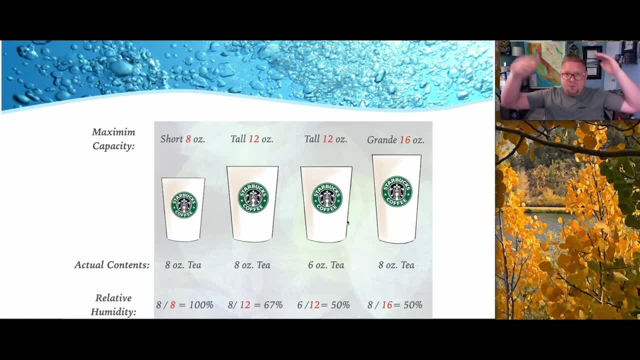 gets more humid, humid, humid, warmer, warmer, humid, humid, and it just keeps getting worse and worse and worse. And that's why there's there have been instances in places you know the South, where they can almost break beyond a hundred percent humidity or break beyond saturation, So it's going to be like 110%. humidity, which means that it is so hot and so humid, but it's still too warm for condensation to occur, So the moisture is literally just floating. So when they say that you can like cut the air with a knife because it's so thick, that's what happens: It's too warm for that, you know. 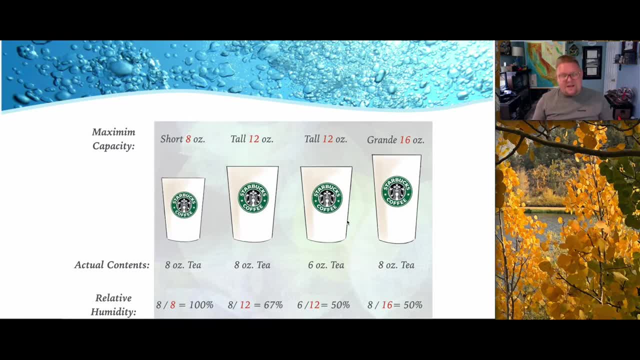 dew point to occur, for it to drop and for it to rain. So instead it's just going to be stagnant and floating and it's going to be really uh. that's why I don't ever go to Disney world, you know, in the summer it's going to be too hot and too humid. I do not do well with humidity And I know. 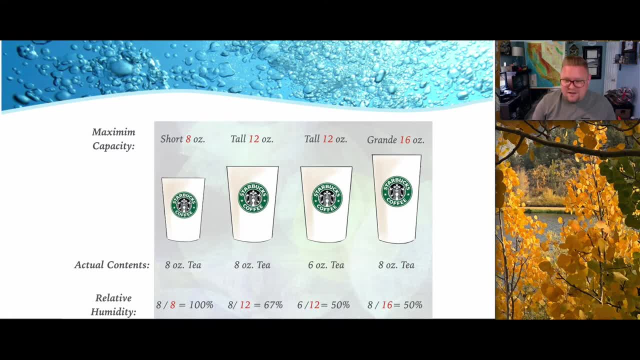 that sounds funny. I always say: that's all well, at least it's a dry heat. I'm telling you, it makes a big difference for me, that idea of uh, of dry heat. So that brings in the values of. 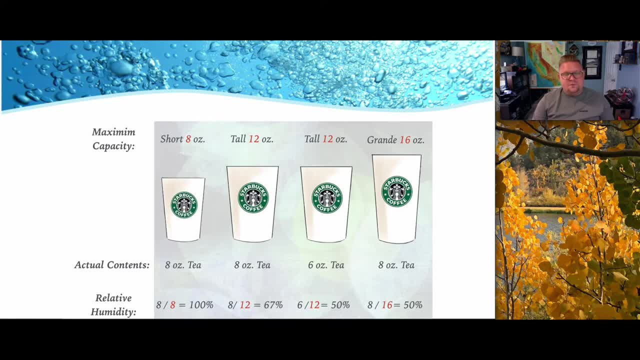 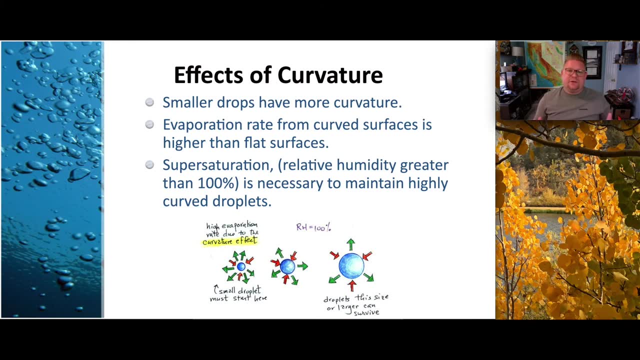 humidity. So the next part we're going to start looking at is: what does that precipitation look like? So we're going to talk about what does precipitation look like, And the first thing that we've got to start off is: are there going to be the effects of curvature? So smaller droplets will have more? 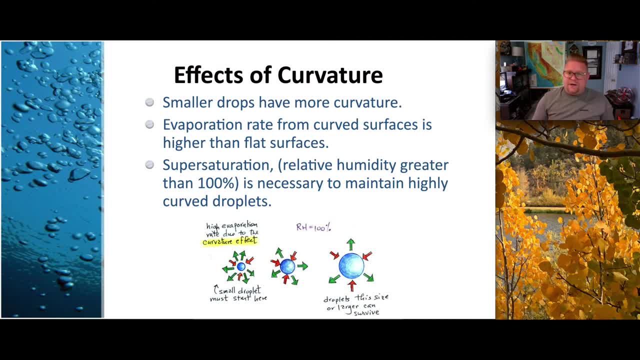 curvature or more shape. Evaporation rate from curved surfaces will be higher than flat surfaces, And this phrase super saturation, which it means relative humidity is greater than a hundred percent- is necessary to maintain highly curved droplets. So we know that humidity is going to be higher than flat surfaces. So we're going to talk about 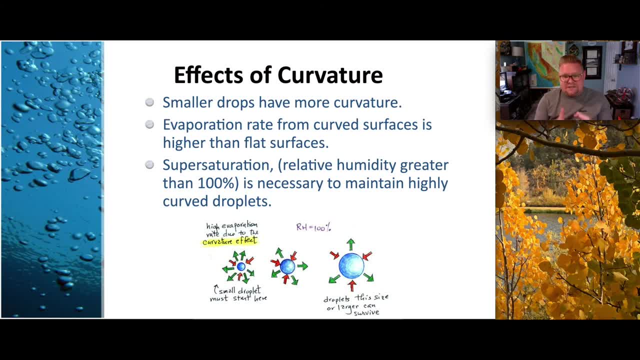 that, We know, that, you know, as a vapor and as it begins to condense into droplets, it's going to be in a shape of a droplet or a circle, but we find that high evaporation is due, you know is caused. 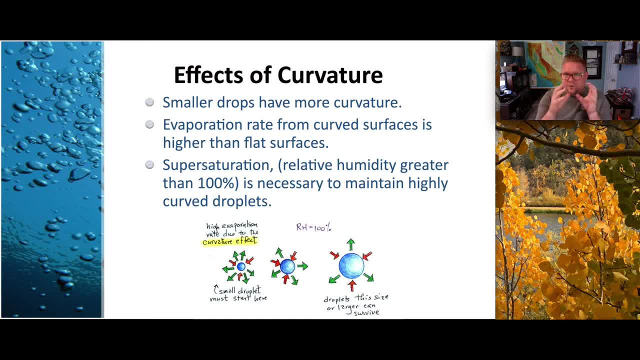 because of this curve, which means that, even though the water droplet can still be in the atmosphere, further evaporation can occur. So what we find is that smaller droplets will slowly become larger. They do so by bumping into other droplets and growing. So it's much like you know thinking. 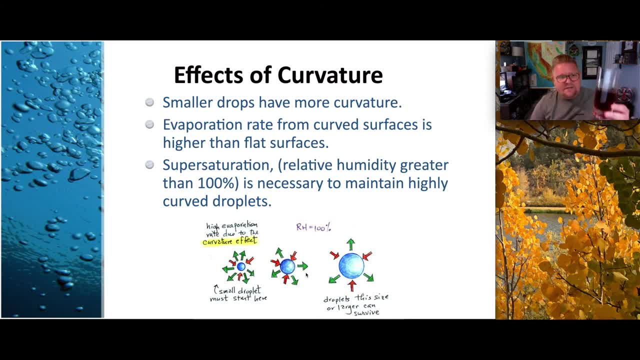 about, like you know, going back to it's been a very popular glass of iced tea. When you have condensation that occurs, then that droplet slowly drips down. As it drips down, it, you know, attaches and grows, with other droplets becoming larger and larger. Well, that's an idea, but 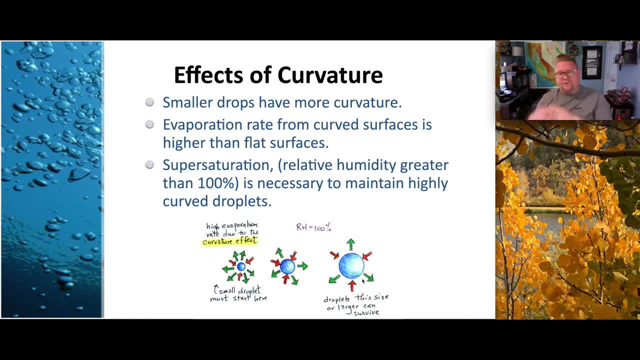 larger droplets are necessary for them to fall and to survive. The smaller droplets will end up just re-evaporating before they even get down to the surface. So that's the first thing. So the effects of curvature, which is something you may not have thought of, that the fact that the shape 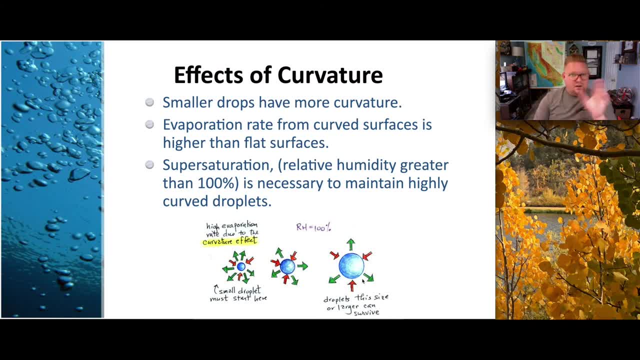 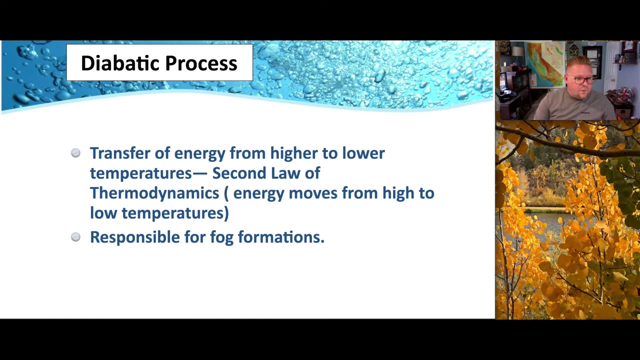 of the droplet plays a role on its process. Again, even in that evaporation, I'm sure that you know that liquid is turning into a vapor. What type of energy is being involved? We've got all this stored energy being passed back and forth. It's really fascinating. Now we do have 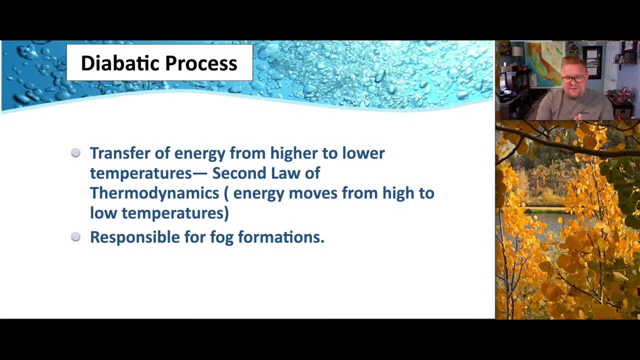 oh, actually before. I'm going to mention this anyway, but as we'll learn more about precipitation in another presentation next, within those droplets and evaporation, we'll also we'll learn that raindrops do not look like the raindrop, that teardrop shape You're going to be. 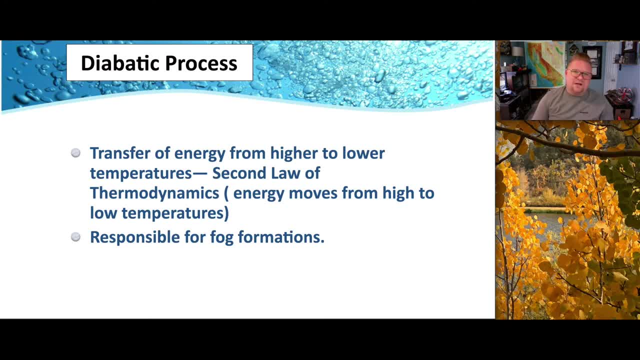 very disappointed. I'm sorry, but that's not actually what they look like And we'll talk about that, But anyway, diabatic processes is a transfer of energy from higher to lower temperatures. It's the second law of thermodynamics: Energy moves from high to low. 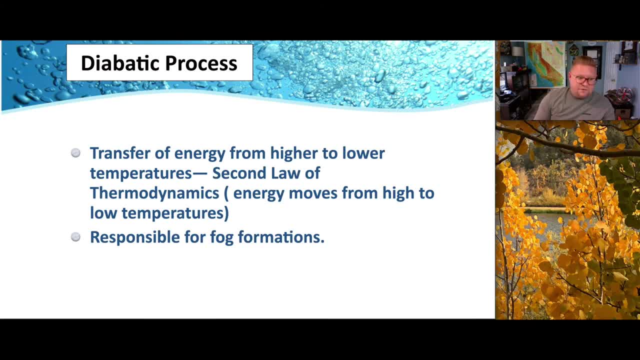 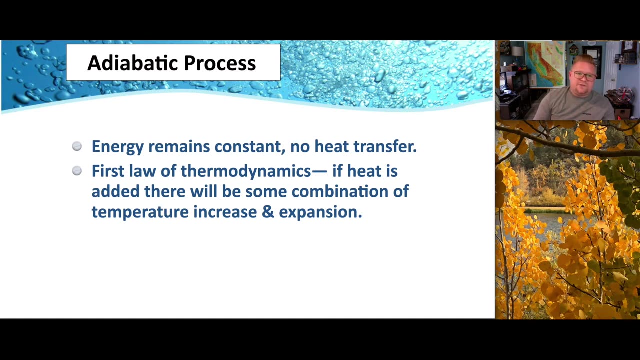 temperatures. It's responsible for many fog formations, which we'll talk a little bit later within fogs, But we have this process. The one that I use the most within my classes is going to be the adiabatic, which is, you know, energy remains constant. There's no heat transfer, It's 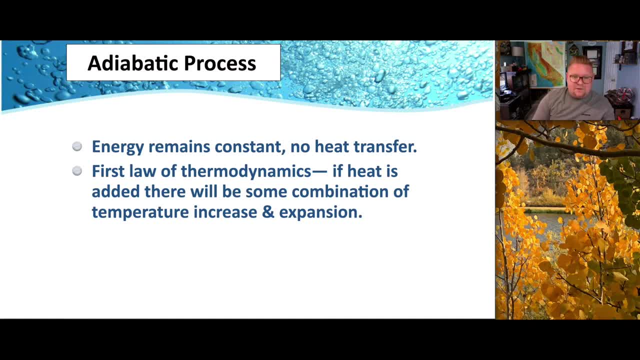 the first law of thermodynamics: If heat is added there will be some, you know, combination of temperature increase and expansion And that we're able to use really these two, you know processes, these two laws of thermodynamics, to look at temperature changes. you know, along mountains. 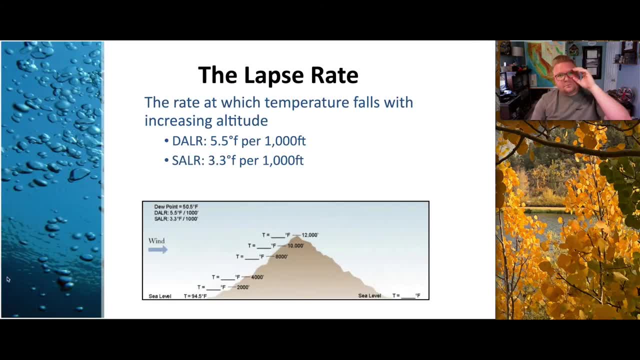 So, as an example- and I've got another video- I'll share the link somewhere up here that teaches you more about the lapse rate and how to calculate it. But essentially here we have a mountain sea level on one side, maybe this: 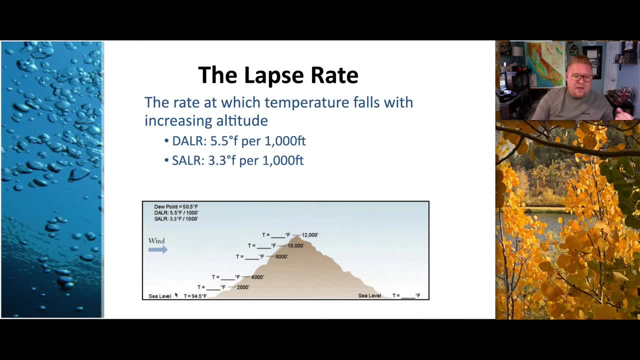 is Santa Monica, Here's the San Fernando Valley on the other, And as we can see, you know, as we go up the mountain, we're going to gain altitude. Well, we learn that, you know, when looking at our atmosphere. you know, especially within our surface, the troposphere is that as we gain, altitude, it continues to get cooler And due to that that you know that notion, we know that the air, the dry air, dry adiabatic lapse rate is about 5.5 degrees Fahrenheit for every 1,000 feet. 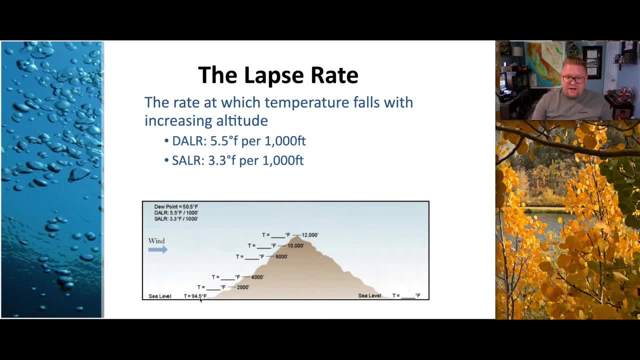 So if it's 94 and a half degrees Fahrenheit on the surface and I hike up 2,000 feet, two times 5.5 is 11.. So it's going to be 11 degrees cooler, 2,000 feet above me. 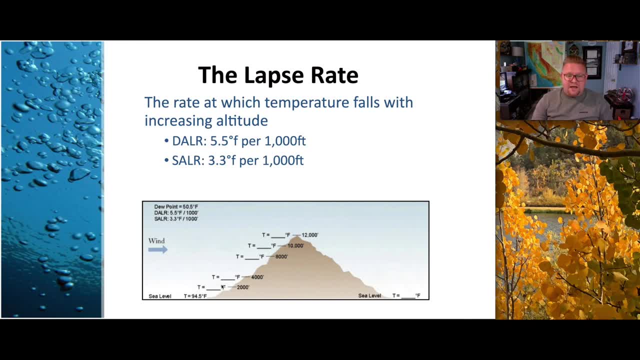 So this is really an interesting, interesting thing. We can look at how temperatures change and then we can actually, you know, if we have a weather station or we're going to do a really big hike, we can actually knowing the 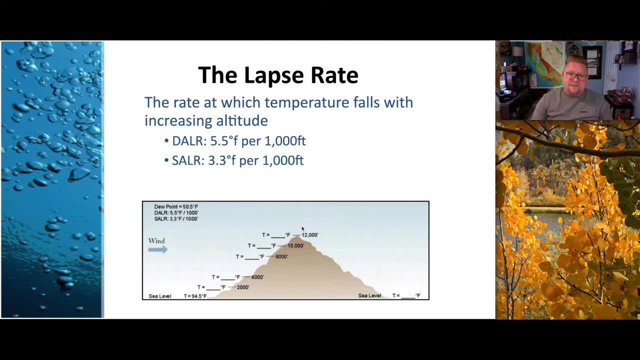 surface temperature, calculate relatively what the temperature at that new altitude would be. So we have another rate, which is the SALR, the saturated adiabatic lapse rate. So we have dry and saturated air. So we end up learning a little bit about the fact that dry air is 5.5,. 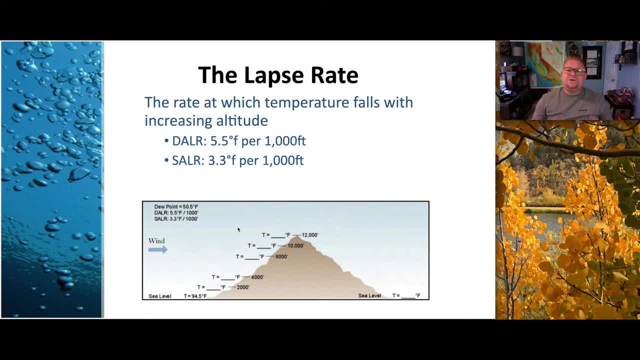 saturated is 3.3.. So saturated means once you hit dew point, once you've hit a temperature that is appropriate for the vapor to condense, the rate of cooling will begin to decrease a little bit. It's not as great. Well, that's interesting because you'd think well. 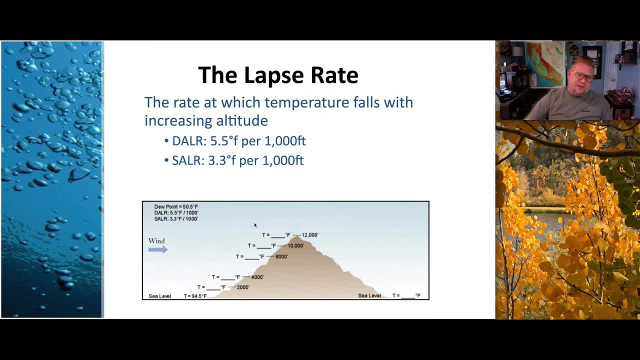 why isn't everything just the same? Why is it that once you hit a dew point temperature, you have to use a different variable? And again, I've got another video that I shared that goes more into depth, but to just very quickly explain it, we're going. 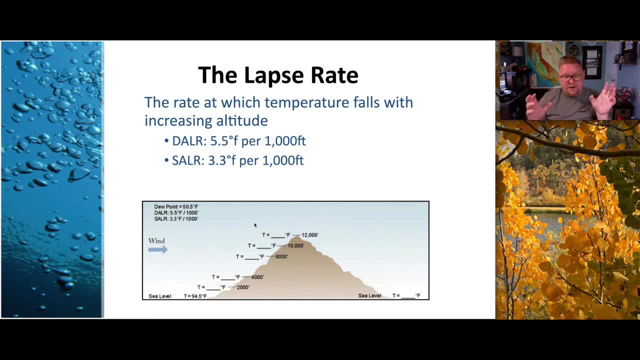 from a vapor into a liquid, right? So condensation is occurring, So we're going from a gas and all of a sudden it's turning into a little bit of a cloud, then it'll turn into rain, right? Well, in that process is energy released or absorbed? And we learned that energy needs to be released in order for it to go from a gas to a liquid, So that 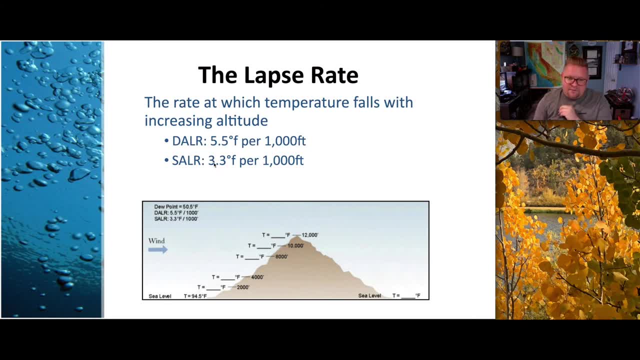 released energy creates a little bit of heat, which really combats this temperature, which is why it actually lessens a little bit. So had that energy not been released, this would have remained a 5.5. But because you have a process that is occurring, that is releasing heat into the atmosphere, it actually causes a slight warming effect, which is really interesting. So there's that part of the lapse right. 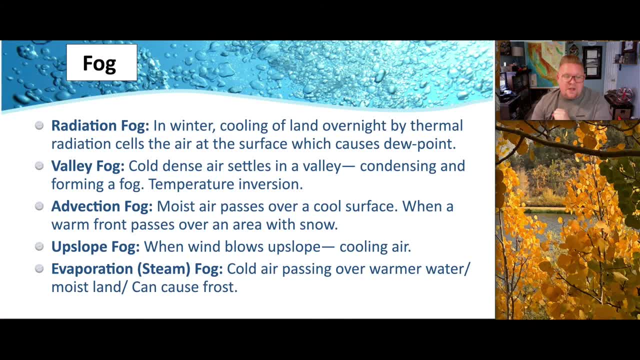 So something else that we've mentioned a little bit is fog, So fog. a friend of mine who teaches Jason Bergdorfer. he has a 70 slide presentation on fog. I have four. I'm sorry to disappoint you. Fog is incredibly interesting and fascinating and absolutely stunning in most landscapes, But there's so much to get through is that I can't spend that much time on it. But we do have observed in this diagram. 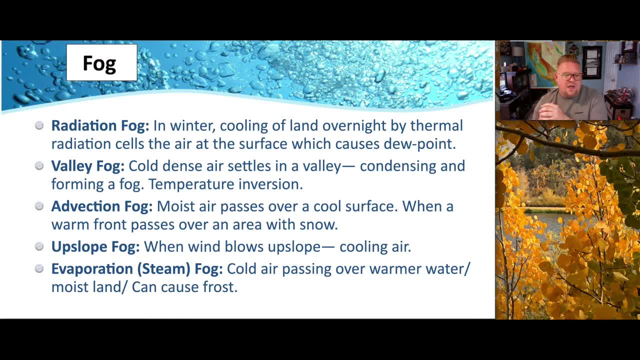 well, in this table five different types of fog On the diagram. I'll share a little bit, actually a six. we'll talk more about what that means. But we have radiation fog, valley fog, advection fog, upslope fog and evaporation, otherwise known as steam fog. 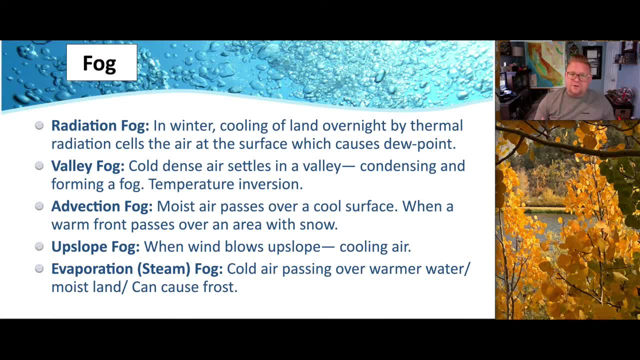 And they all operate differently. so radiation, you know, in the winter, cooling of, you know of the land overnight by thermal radiation cells, the air at the surface will cause dew point to occur. valley fog is when cold, dense air settles within the valley, condensing and forming a fog there, known as temperature inversion. advection is moist. 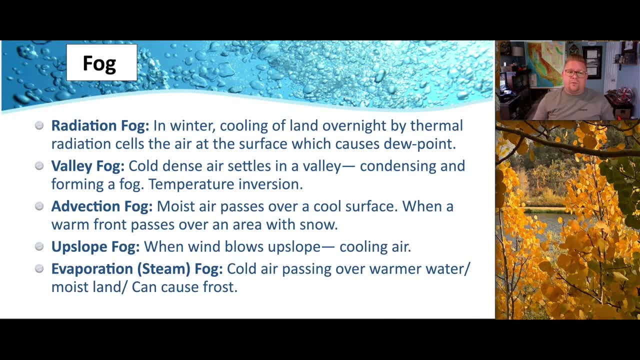 air will pass over a very cool surface when the warm front passes over it and will bring in, bringing in snow, essentially upslope fog. when the wind blows upslope, so it forces it upward and it, you know, causing it to cool and will create a fog and then evaporation, which is cold air passing over a much warmer 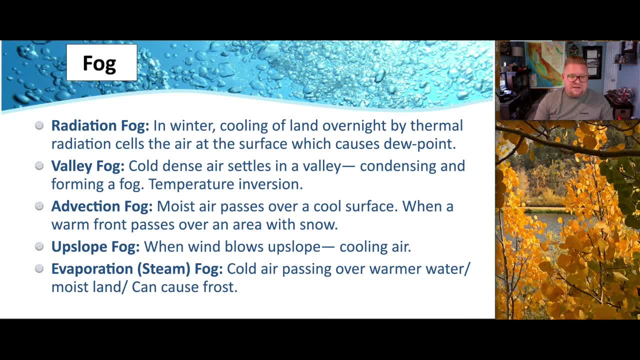 landscape. it can also cause frost. I've seen when I live in Santa Clarita- and we do, I as a kid, all the farms, the hot summer days, you know in the morning, all day long, that energy is absorbed, radiation at the surface and it gives off that heat and it gives it off during. 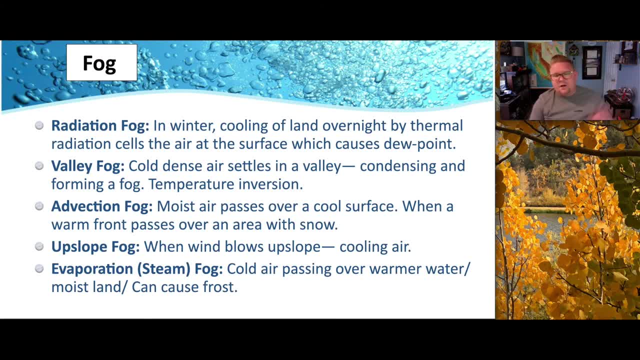 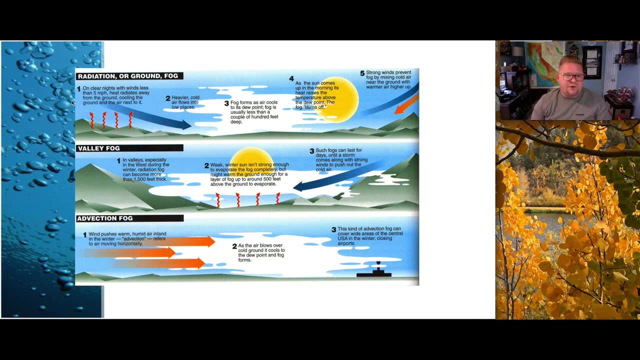 the middle of the morning the next day, and so that cooler air comes in and you can actually see the steam coming off the surface, which is really interesting. so what did these look like? so here are some diagrams, going into further definitions, so you, as an example, radiation or ground fog- you know the 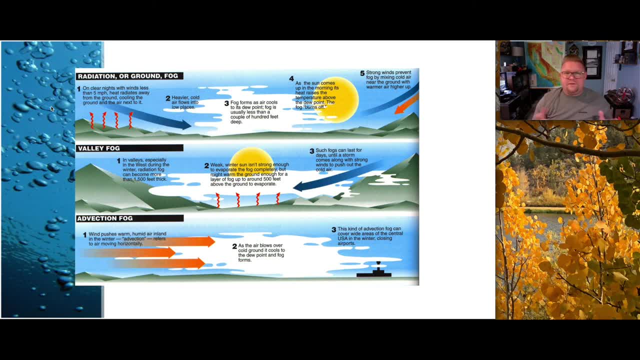 first step: on a clear night with winds less than five miles an hour, the heat will radiate away from the ground. you know the first step: on a clear night with winds less than five miles an hour, the heat will radiate away from the ground, cooling the ground because that heat is transferring away, then a heavier cold. 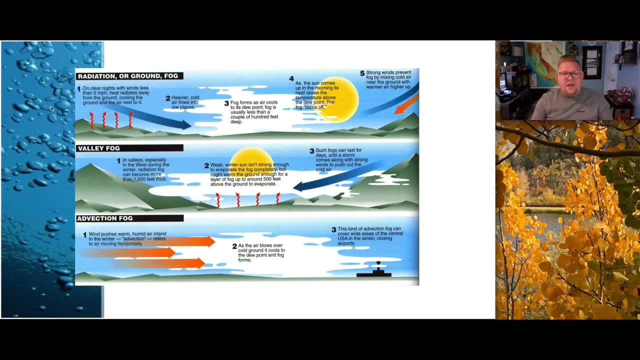 air flow will bring in low, you know, into low- air. step three: fog will form as the air cools to its dew point. fog is usually less than a couple hundred feet in depth. step four: as the Sun comes up in the morning, its heat raises the temperature above the dew point and then burns off the fog, and so you have these. 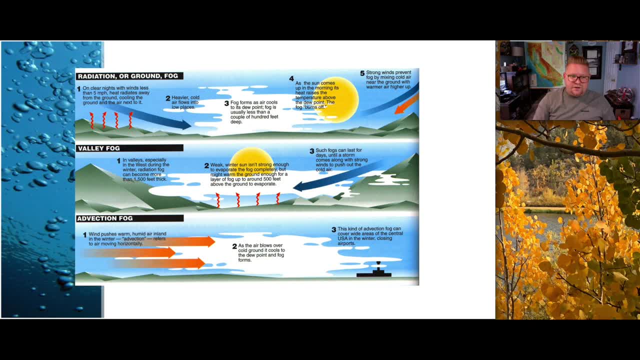 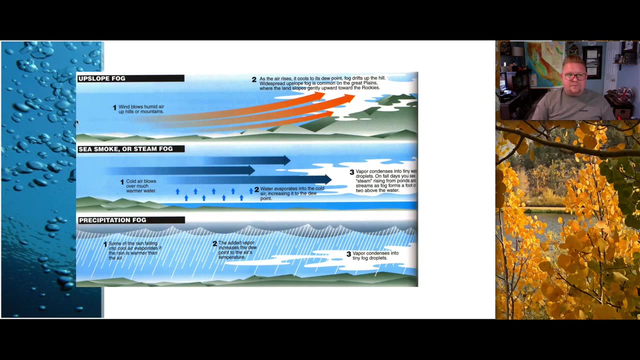 processes. so here we have again radiation. here's an example of Valley fog and we have convection fog. so leave that there because you want to like take a screenshot or pull that up. and then the last three. we've got upslope, we've also got smoke or steam fog, which I mentioned. the last one is 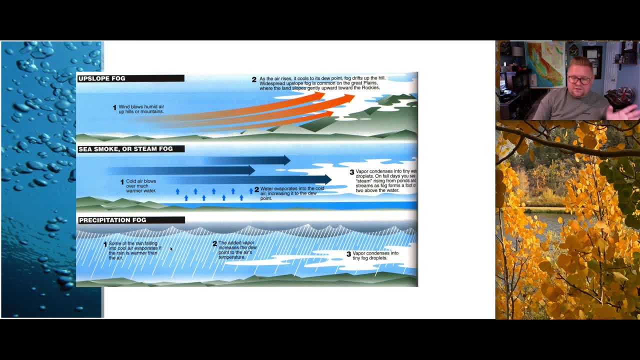 precipitation fog. that was not on the earlier slide, but I like this diagram that was very helpful, showing that some of the rain falling into cool air will evaporate if the rain is warmer than the surrounding air and that added vapor will increase the� increase the dew point to the air's temperature and then the vapor will condense into tiny fog. 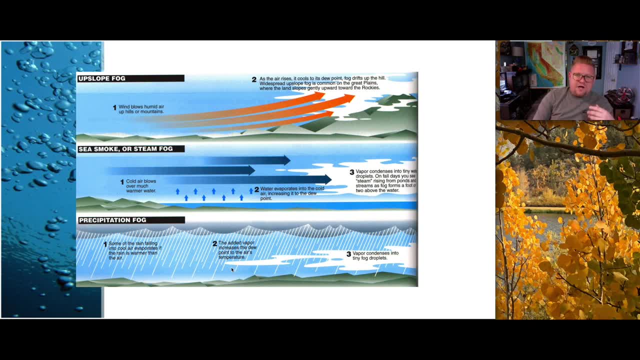 droplets. that's a really interesting one. it's very different that it's not as commonly studied as the other five that i presented to you earlier, but it is something else to work through. so again, we've got these, you know, five major way of fogs that can be observed and interpreted on our 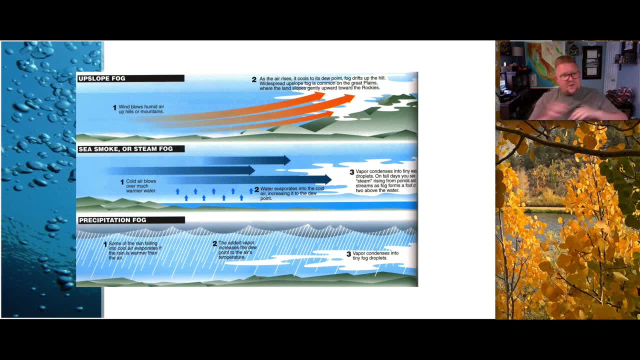 landscape. um, again, this is just the introduction to atmospheric moisture and fog. you know there's so much more that can be covered with your texts and other resources, but this is kind of painting that picture of some of the key terms, how they work, how they operate and how we continue to use.